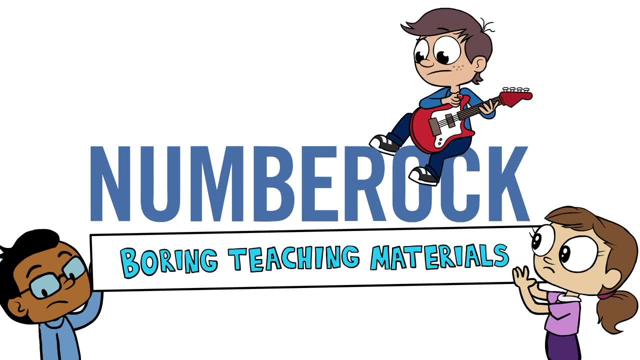 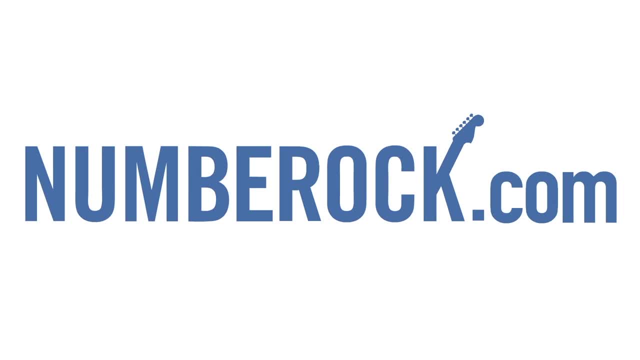 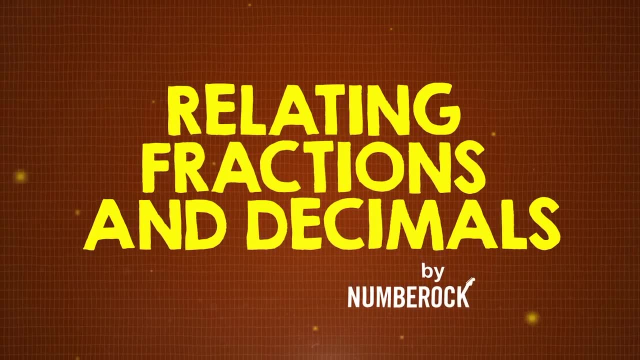 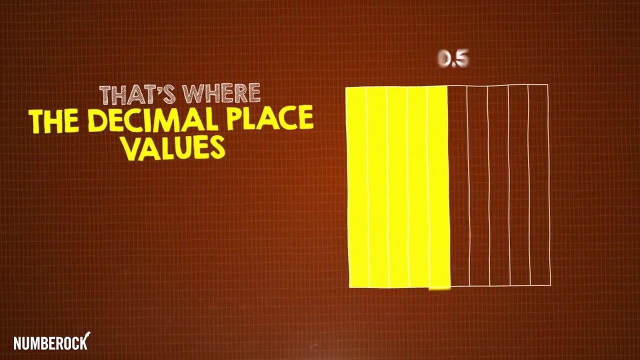 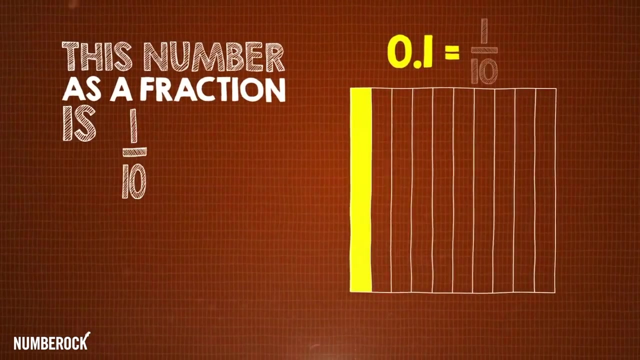 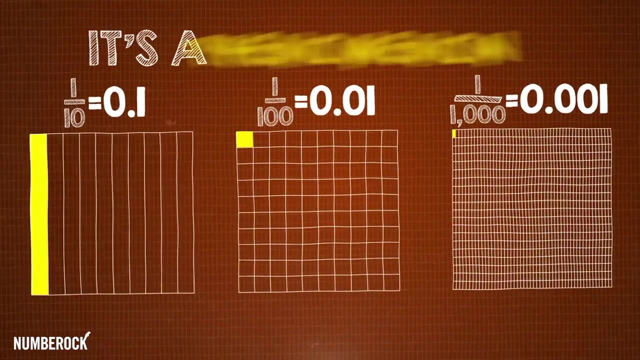 Get on over to NumberRockcom for some very not boring teaching materials And ad-free videos, NumberRockcom. This number as a fraction is 1 over 10 and 0.1 is its decimal equivalent. Fractions over 10, 100, 1000 and on are all decimal numbers. it's a phenomenon. 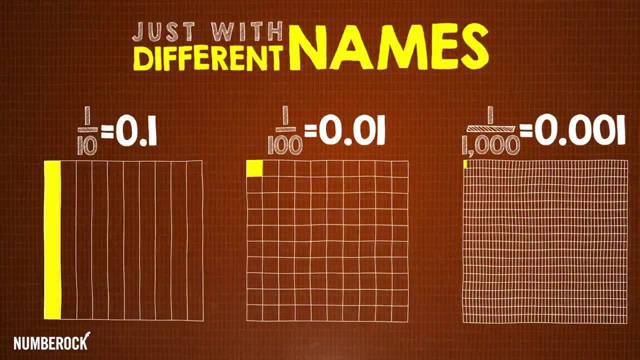 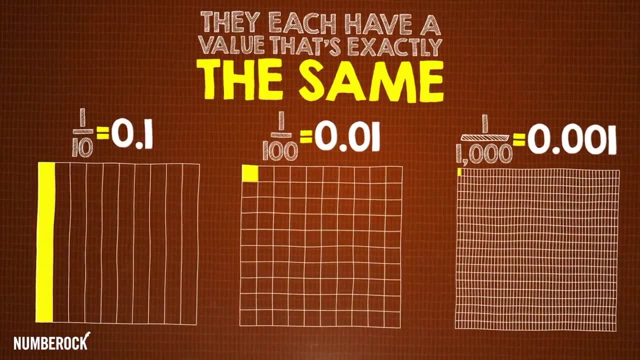 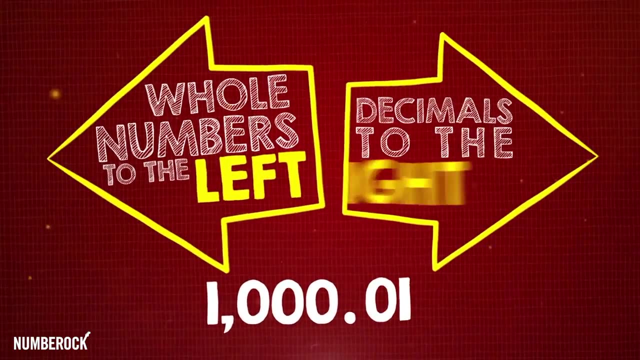 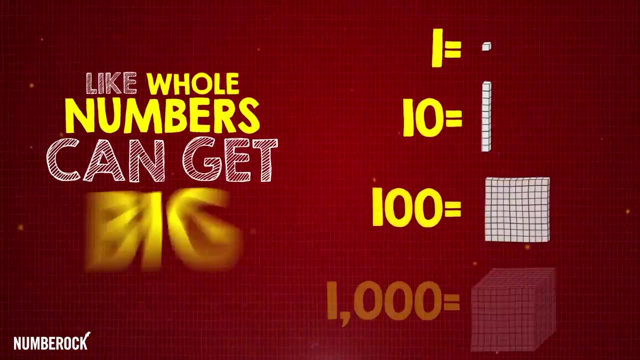 Decimals are fractions, just with different names. They each have a value. that's exactly the same. Whole numbers to the left, decimals to the right. They get smaller and smaller Till they're barely inside Like whole numbers can get big. decimals can get small. 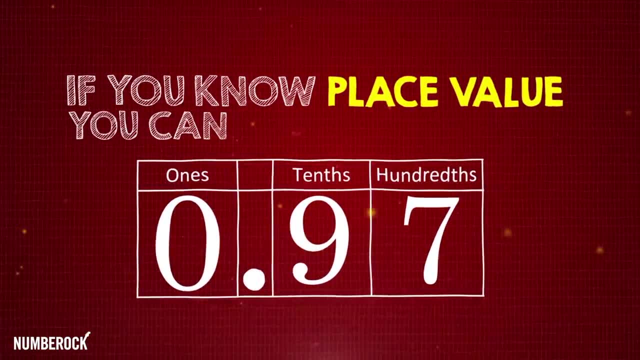 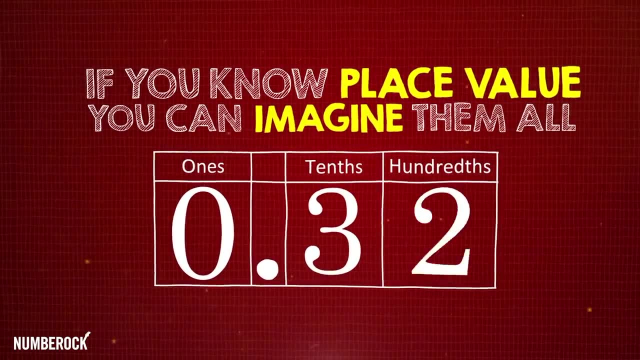 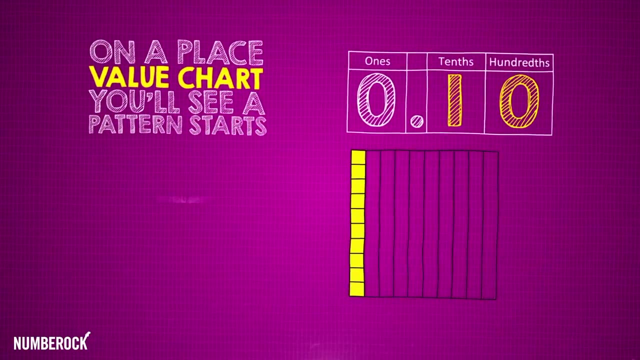 If you know place value you can imagine them all On a place value chart. you'll see a pattern starts. If you split 1 tenth into 10 equal parts, this new value is 1 hundredth And in every case 100 hundredths. 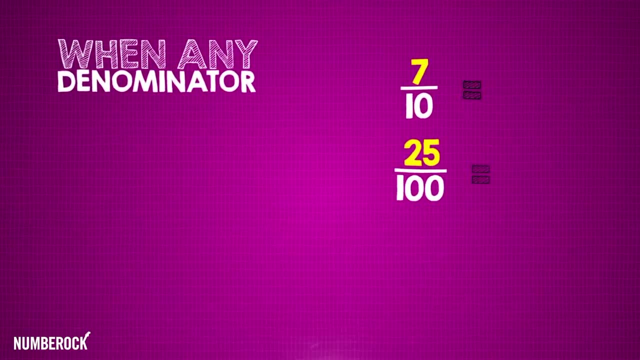 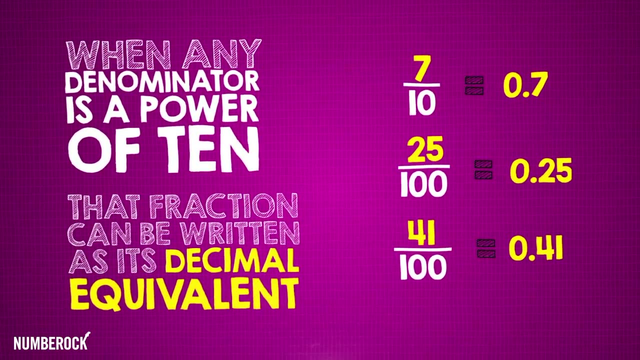 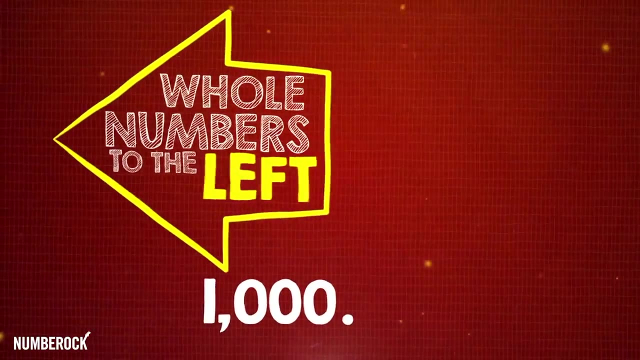 So 1 hundredths equals 1 whole and the ones place When any denominator is the power of 10. That fraction can be written as its decimal equivalent. Whole numbers to the left, decimals to the right. They get smaller and smaller. 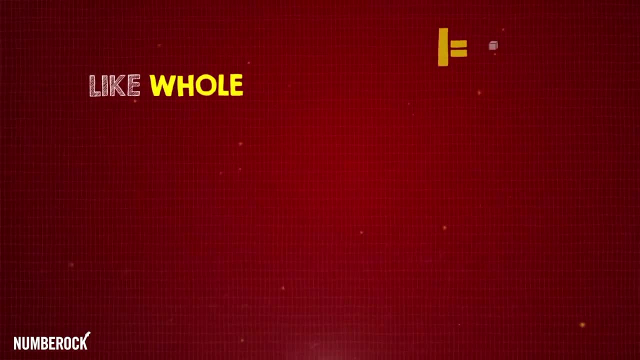 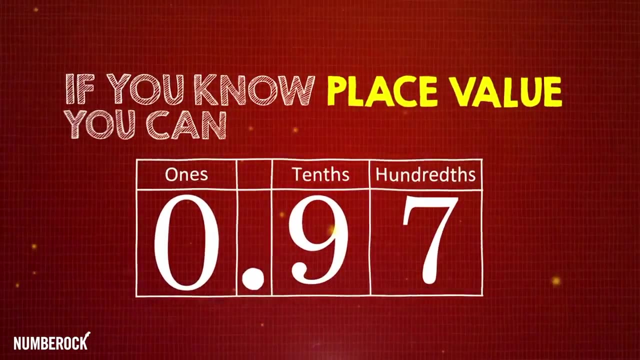 Till they're barely inside. Like whole. numbers can get big. decimals can get small. If you know place value, you can imagine them all. Decimals can't get small. if you know place value, you can imagine them all. We've got the tenths, the hundredths, the thousandths and more. 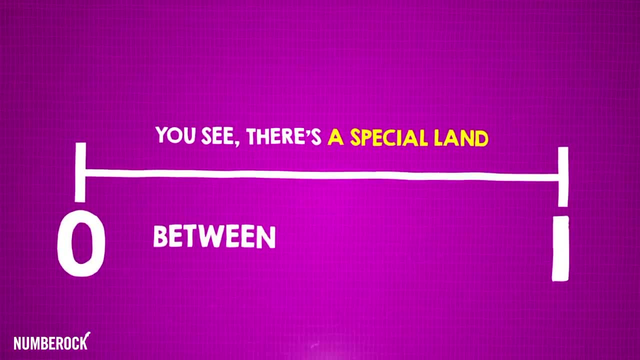 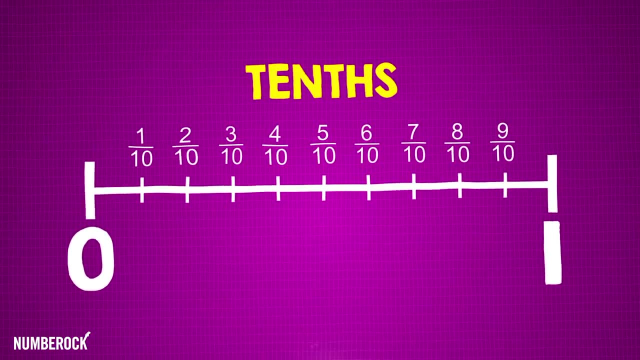 Let's imagine a number line to further explore. You see, there's a special line between zero and one where you'll find decimal numbers In every fraction between zero and one make ten intervals. These are tenths written as fractions or decimals. 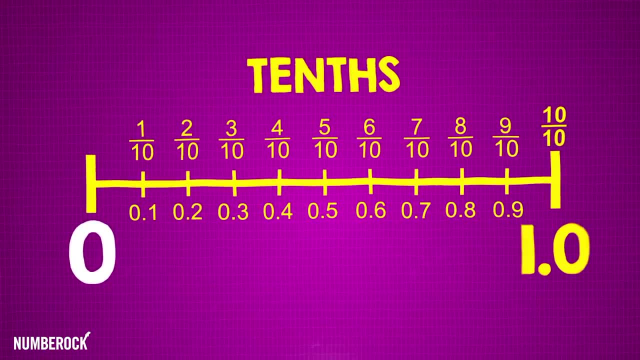 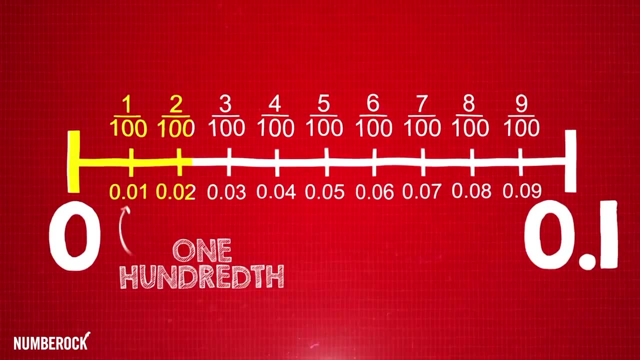 When counting by tenths after you get to nine, the tenth tenth makes one hole on the number line. Let's see what happens as the place value decreases. And when tenth is divided into ten equal pieces, we get a hundredth written as point zero one.